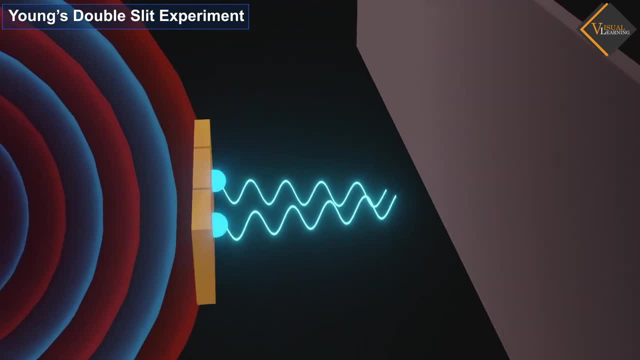 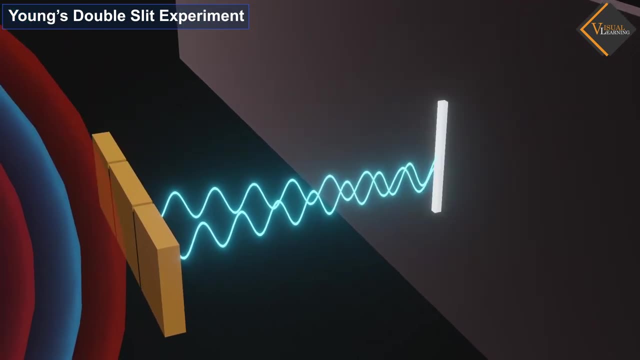 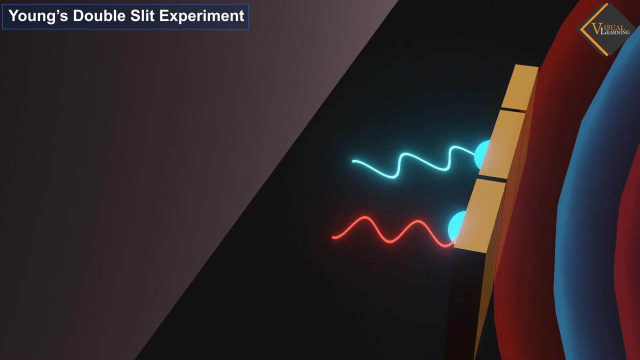 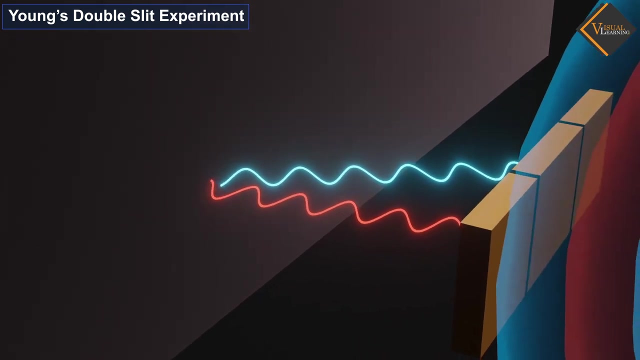 Additionally, it was observed that light waves exhibit interference where two or more light waves superimpose on each other, resulting in constructive or destructive interference. This phenomenon is known as interference. Now let's understand this experiment into details. To understand this experiment, we need to understand some basic terms. 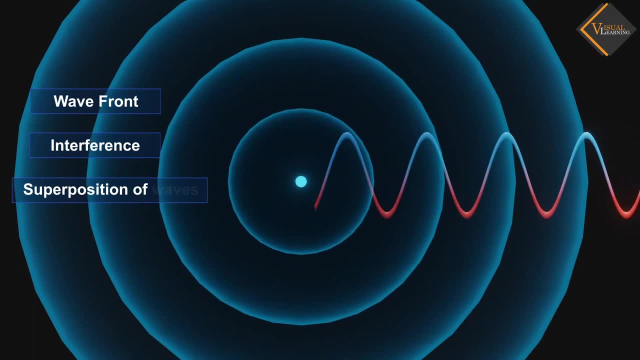 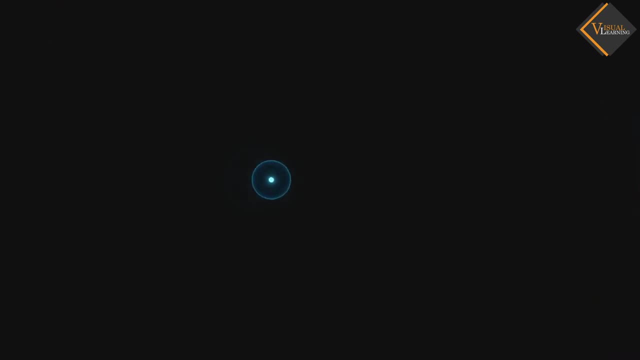 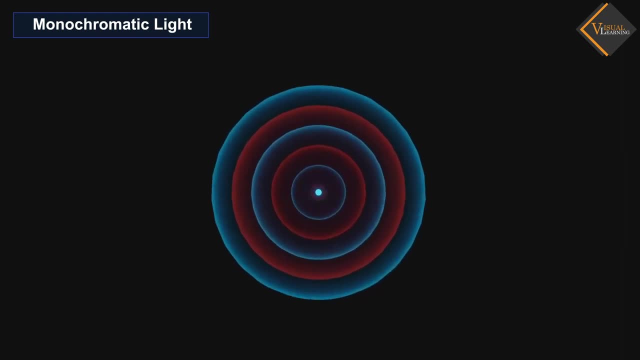 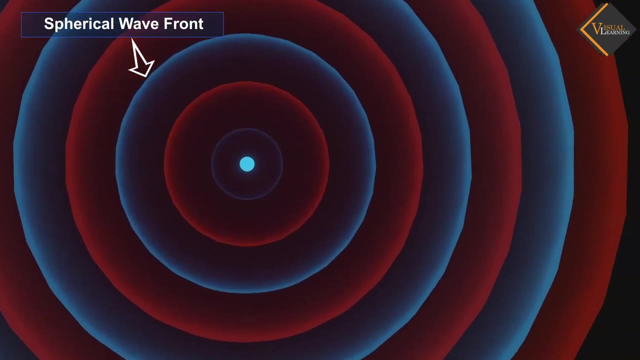 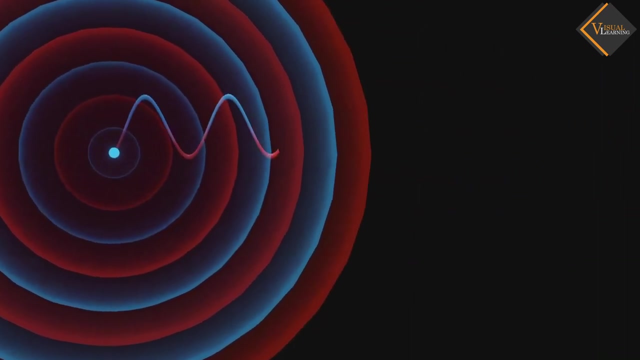 Monochromatic light sources emit single-color light. These light waves are emitted in the form of spherical wave fronts. In general, light waves emit light in the form of spherical wave fronts. These light waves are represented as sine waves, But in three dimensions they travel in the form of spherical wave fronts. 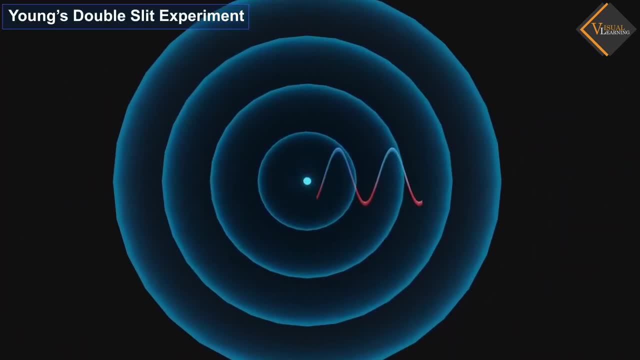 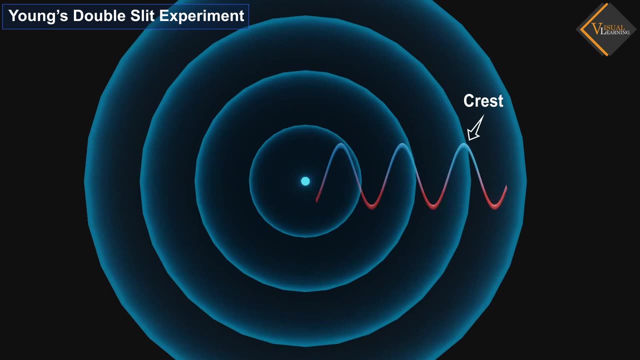 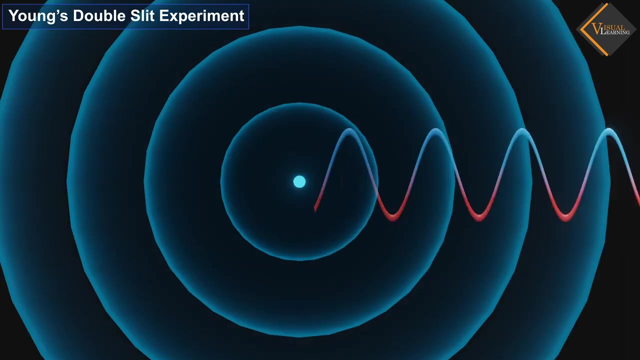 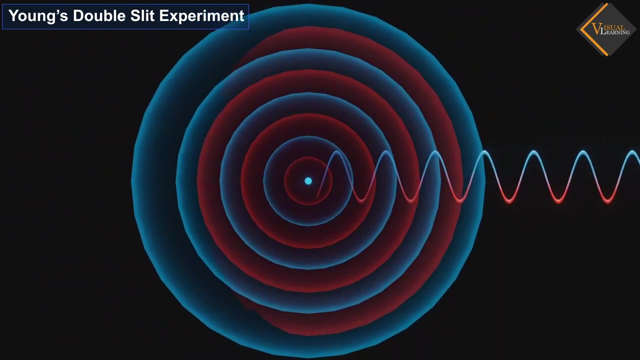 We can consider the surfaces of these wave fronts as wave crests, representing the maximum intensity of the light wave, and the areas between two spherical wave fronts as wave troughs, representing the minimum intensity of the light wave In this light wave. we will consider the blue spherical wave front as the crest. 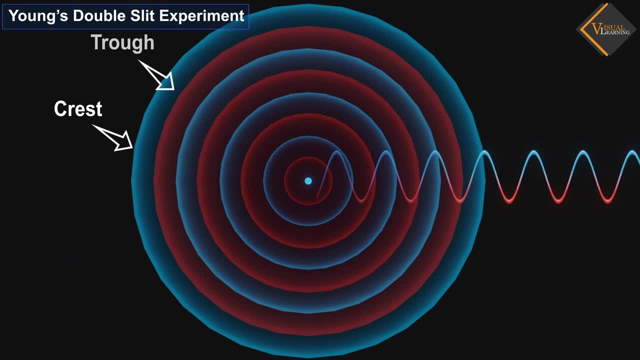 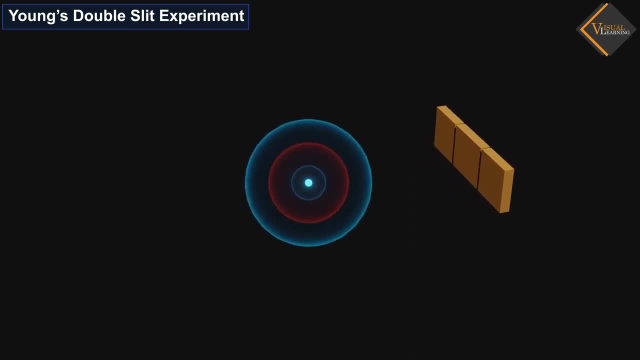 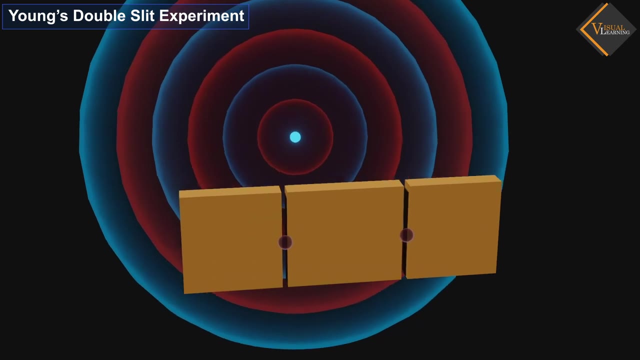 and the red spherical wave front as the trough In the animation we see that when these spherical wave fronts move away from the source, the radius of the waves increase. Now consider: there are two slits placed in front of these light waves, with very sharp openings allowing the light wave to move away from the source. 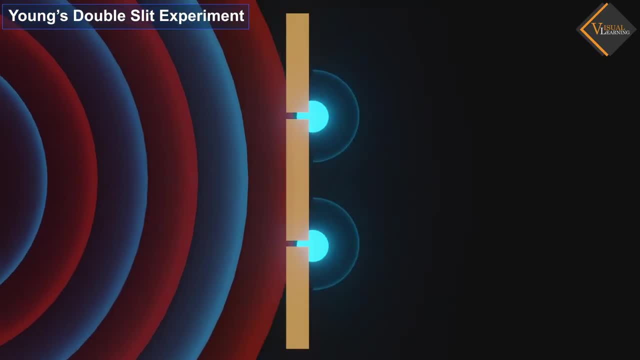 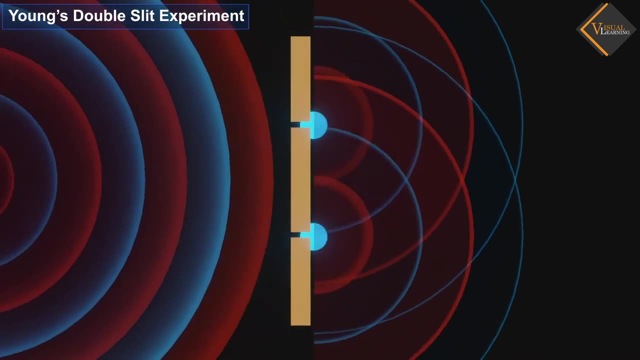 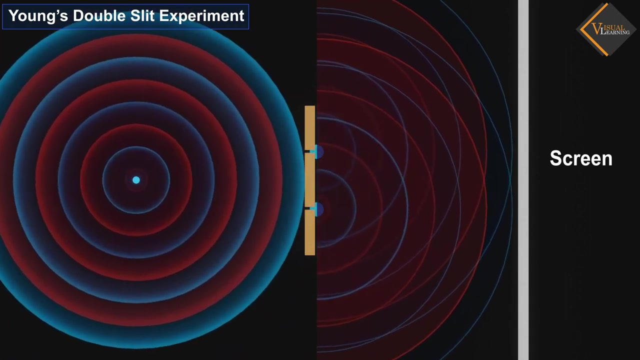 When these light waves encounter the slits, two new light sources are created at the slits, generating new light waves. These light waves are incident on the screen and create a pattern like this. We refer to this light pattern as interference fringes.